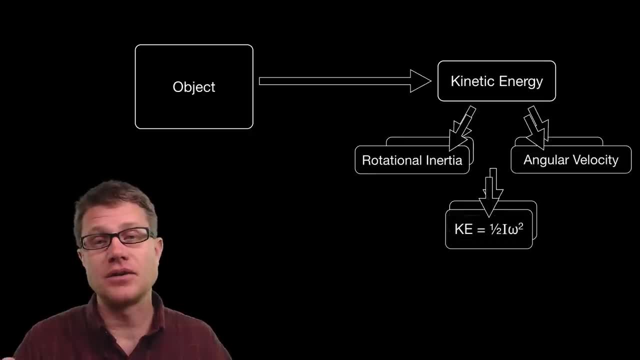 it still has rotational kinetic energy, And instead of using mass and velocity, we are using its moment of inertia, or rotational inertia, instead of mass, And then we are using its angular velocity. You can see, the equation is essentially going to be the same thing. 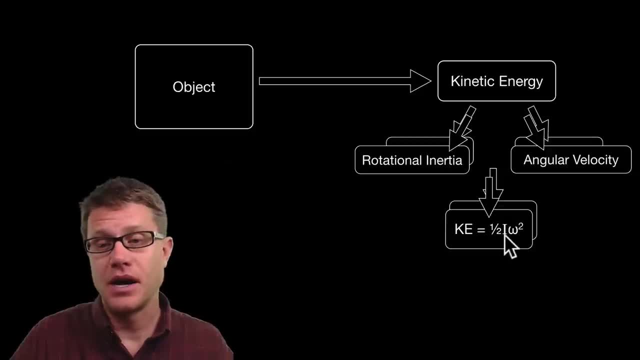 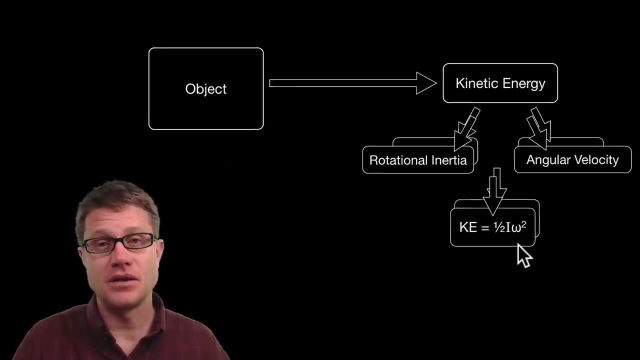 Now, kinetic energy is 1 half i omega, squared where i is rotational inertia and omega is going to be the angular velocity. But remember, this does not have potential energy if it is in motion. We can only have potential energy if there is another object or another part. 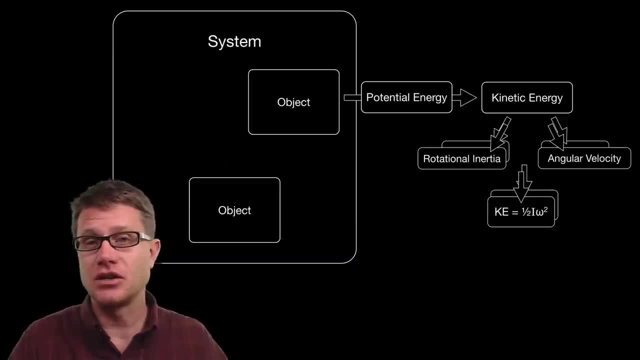 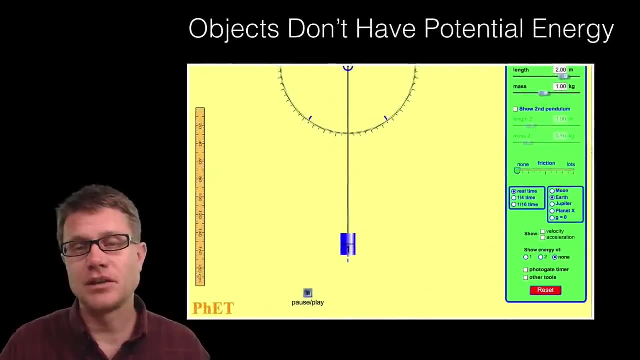 of this system, Then it can have potential energy. It could be gravitational, It could be electric potential energy. But remember, objects by themselves do not have potential energy. And let me use a little PHET simulation to get at that. So if we take a pendulum and 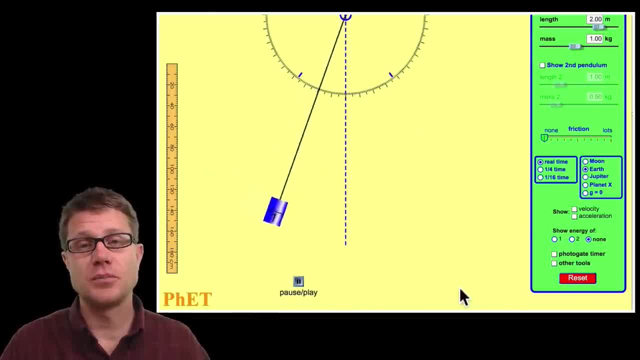 we lift it up on the earth, it is going to have potential energy, which becomes kinetic and then becomes potential energy again. It is going to oscillate back and forth. But watch what happens if I get rid of the earth Now. there is no gravity and I simply let it. 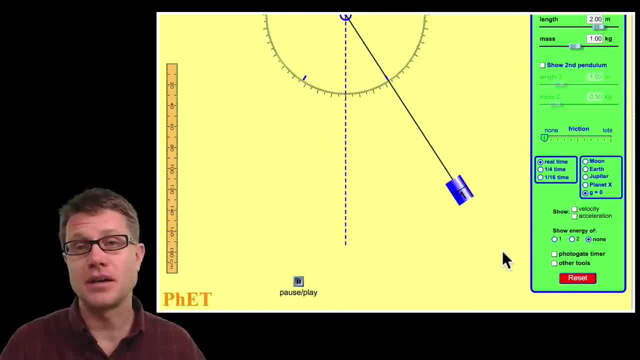 go. Well, that object is going to stay there. It has no potential energy, There is no stored energy because it is a single object. Let me add the earth again. Now we have added that potential energy back, Let's say I pull the earth away. What happens Now? all that energy is just in kinetic energy or energy. 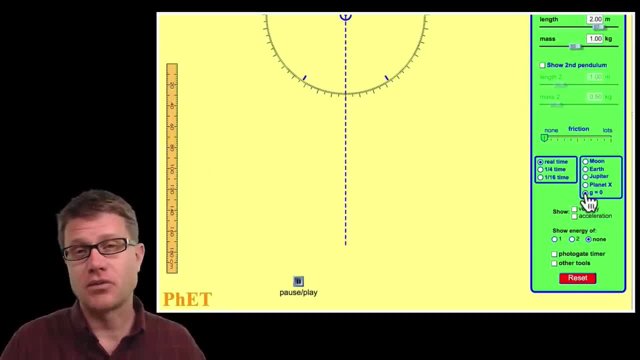 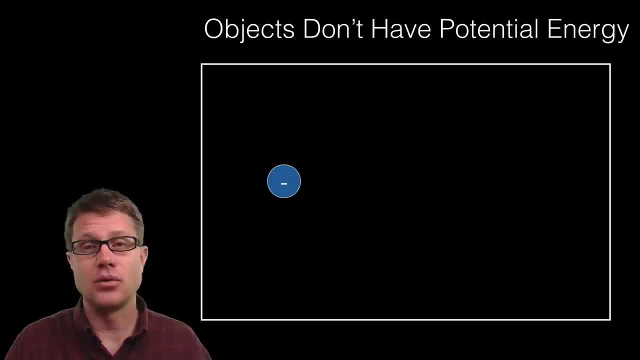 of motion. It is just going to keep moving like that, And so this is gravitational potential energy, But remember, we could have electric potential energy as well. If we have a single charge like this, then there is going to be no potential energy, But if I add other objects, 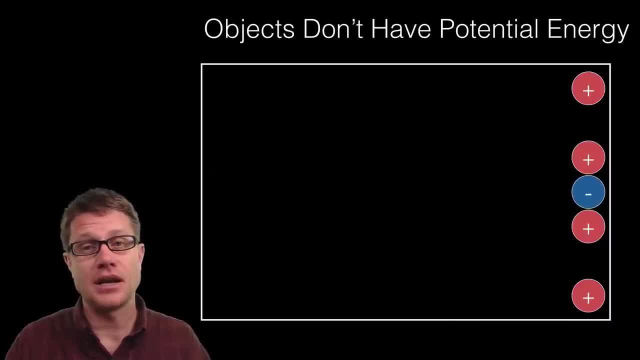 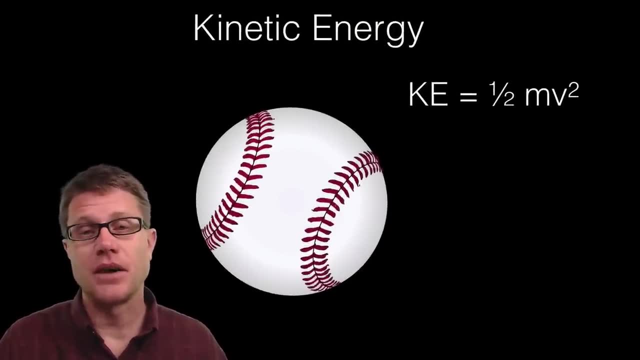 then we can convert some of that electric potential energy into kinetic energy. And if we know the mass of the object and the velocity we can figure out its kinetic energy. The equation is pretty straightforward. If I were to pitch a baseball at around 90 miles. 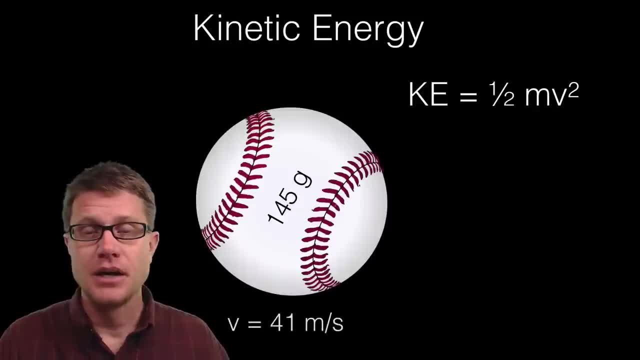 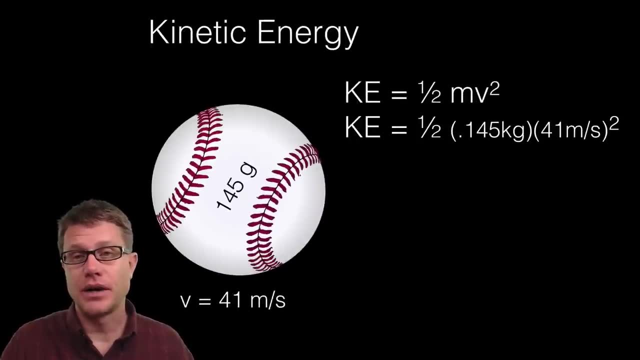 an hour. So a baseball weighs around 145 grams, 90 mile an hour. pitch is going to be 41 meters per second. So I essentially add those values to my equation, And so it is one half 0.145 kilograms. Remember, we have to convert grams into kilograms. And then I have got my meters.